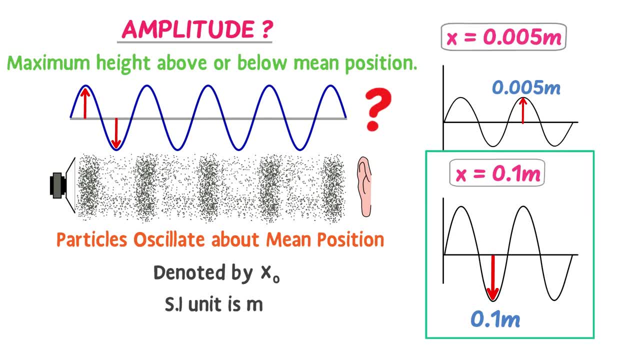 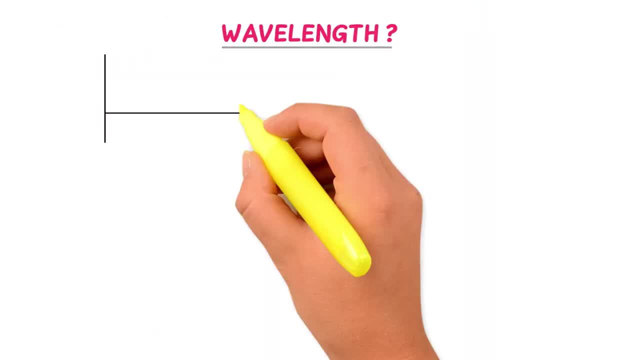 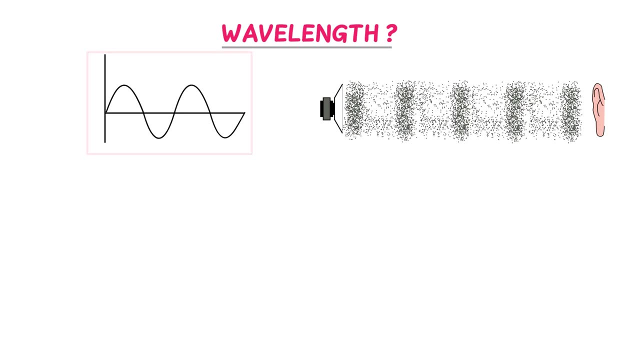 the amplitude of this wave is smaller than the amplitude of this wave. Now, what is wavelength? Well, consider the motion of this wave. We know from the previous lecture that transverse waves travel in consecutive or successive crest and trough, while longitudinal waves travel in successive compression and rarefaction. 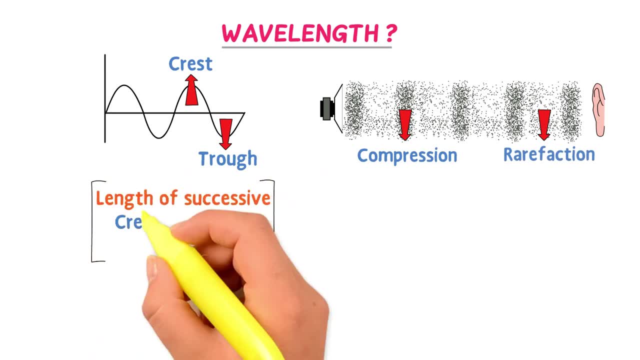 In case of transverse waves, the length of successive crest and trough is called its wavelength, While in case of longitudinal waves, the length of successive compression and rarefaction is called its wavelength. Wavelength is denoted by the Greek letter lambda. Its SI unit is meter. 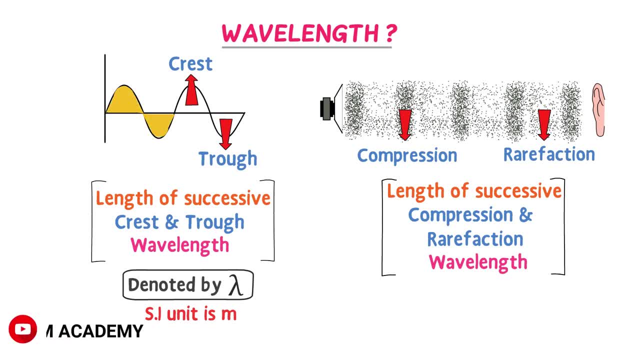 We know that this region is crest and this region is trough. So the length of one crest and one trough is wavelength or lambda. Let's suppose that its wavelength lambda is equal to 0.01 meter. So lambda is the wavelength and one trough is the wavelength. Now let's 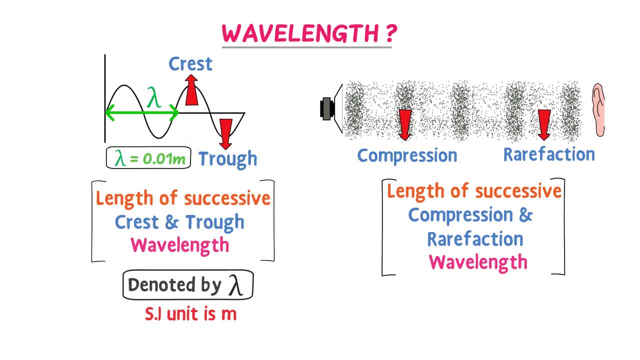 0.01 meter. We also know that this region is compression and this region is rarefaction. So the length of one compression and one rarefaction is wavelength or lambda. Let's suppose that its wavelength, lambda, is equal to 0.002 meter. Thus, remember that wavelength is the length of successive crust and trough. 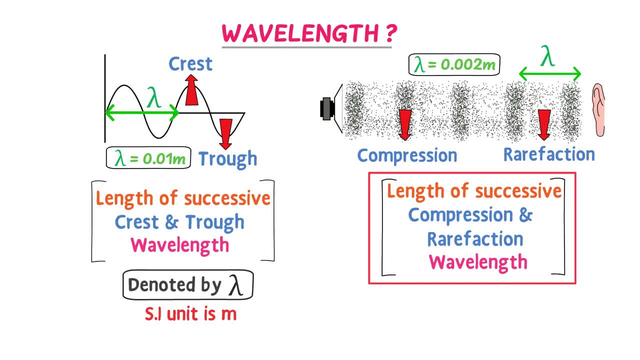 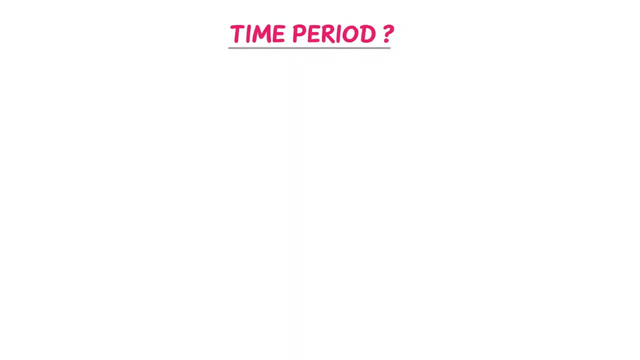 Or it is the length of successive compression and rarefaction. Now, what is time period? To understand the concept of time period, you must understand the concept of wave cycle. Let's consider the motion of these two waves. In case of transverse waves, one crust and one trough form one wave cycle or one. 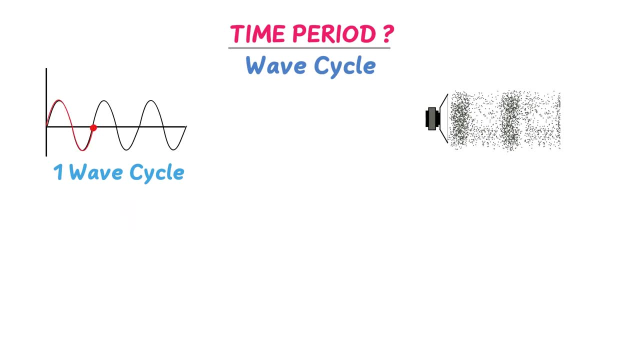 oscillation, While in the case of longitudinal waves, one compression and one rarefaction form one wave cycle or one oscillation. Now, how many wave cycles or oscillations are there? and transverse waves, And how many wave cycles or oscillations are there? and 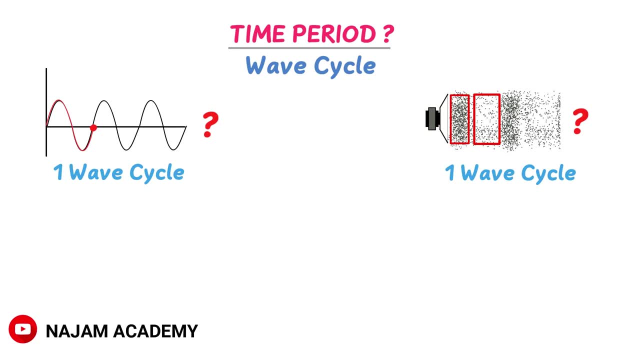 longitudinal waves. Well, this crust and trough make one wave cycle, This crust and trough make another wave cycle, And this crust and trough also make another wave cycle. So there are three wave cycles or three oscillations in this transverse wave motion. Here this compression. 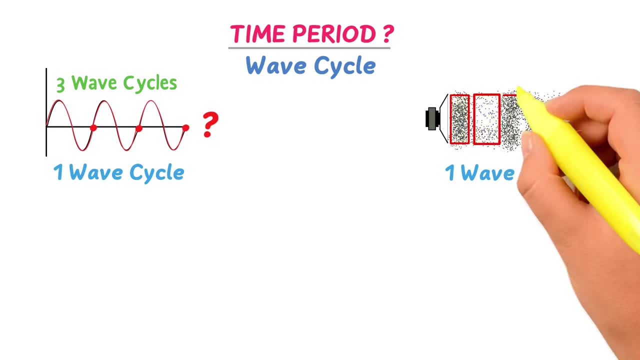 and rarefaction make one wave cycle And this compression and rarefaction make another wave cycle. So there are two wave cycles, are two oscillations and this longitudinal wave motion. Now listen carefully. Time period is defined as time taken by the oscillating body. 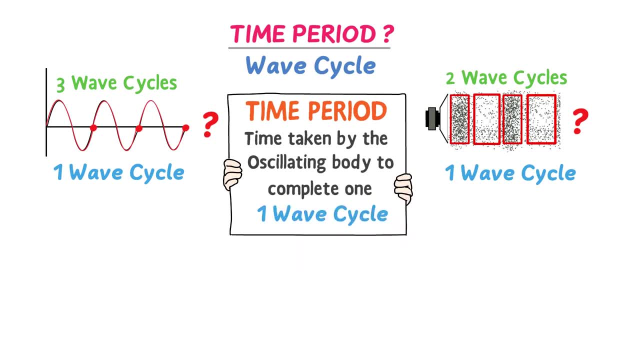 to complete one wave cycle or one oscillation. Let me repeat it: Time taken by oscillating body to complete one wave cycle or one oscillation is called time period. Time period is denoted by capital T and its SI unit is second. For example, if this wave completes its one oscillation or one wave cycle. 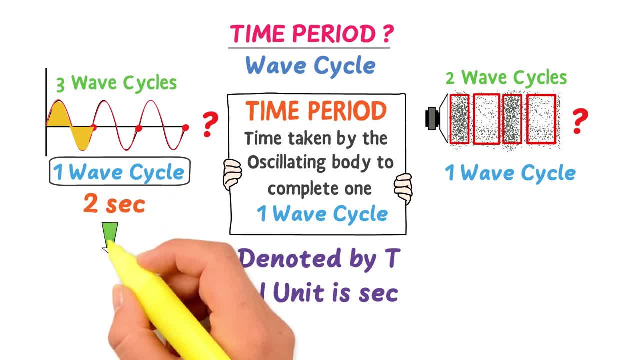 and two seconds, then its time period is T is equal to two seconds. If this wave completes one oscillation or one wave cycle and one second, then its time period is T is Thus: remember that time period is the time taken by oscillating body. 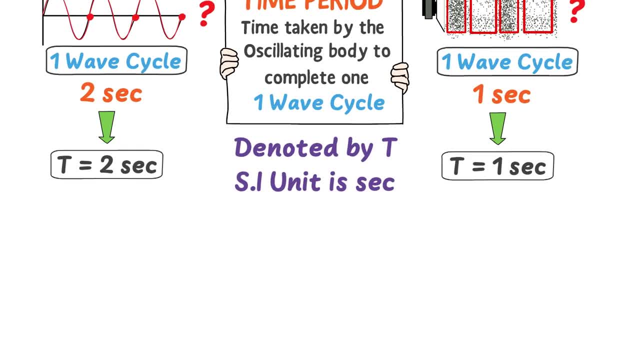 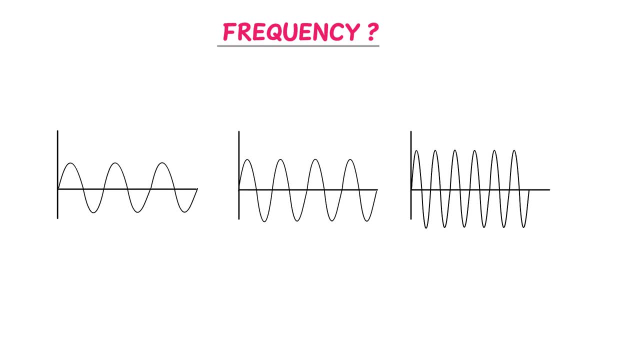 to complete one cycle. Finally, let me teach you that what is frequency? Well, consider the motion of these three waves. Let in one second, this wave completes three wave cycles, or three oscillations. This wave, in one second completes four wave cycles. 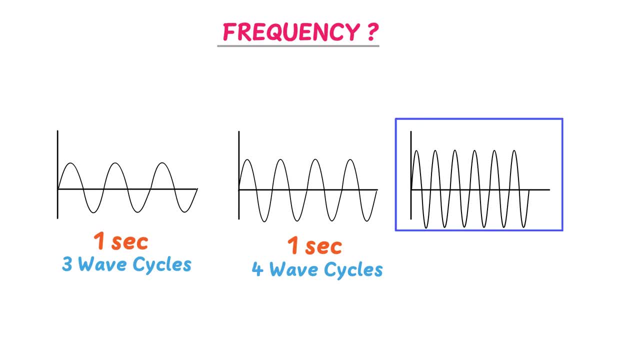 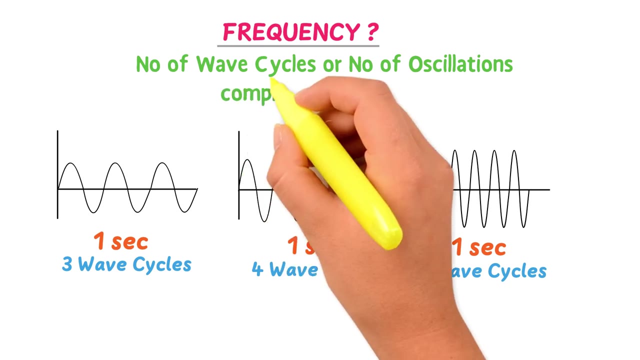 While this wave in one second completes six oscillations or six wave cycles, We define frequency as number of wave cycles or number of oscillations completed in one second. Let me repeat it: Number of wave cycles or number of oscillations completed in one second.